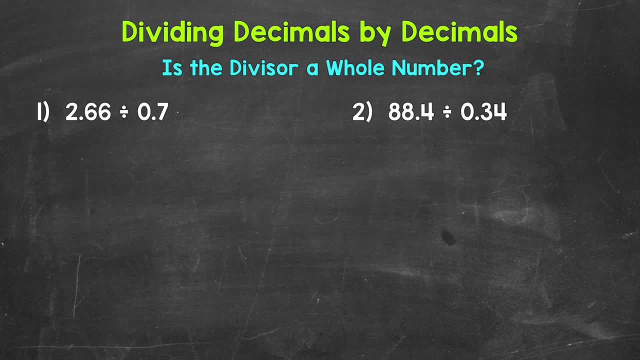 divided by 7 tenths. The first thing that we need to do is set this problem up. That way we can go through the division process. 2 and 66 hundredths is the dividend, the number we are dividing. It goes under the division bar. 7 tenths is the divisor, the number we are dividing by. 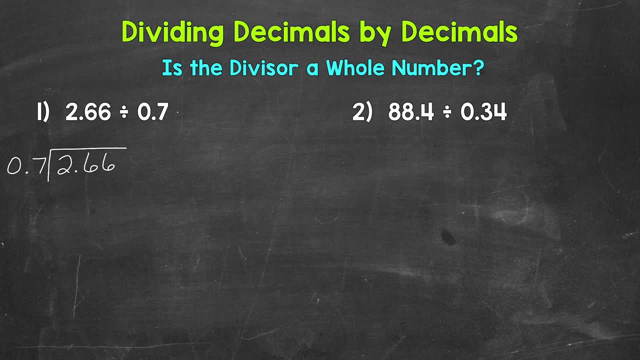 It goes on the outside of the division bar. Now, whenever we have a division problem that involves decimals, we always need to check: Is the divisor a whole number? Well, 7 tenths is our divisor. That's not a whole number, So we need to make it a whole number. 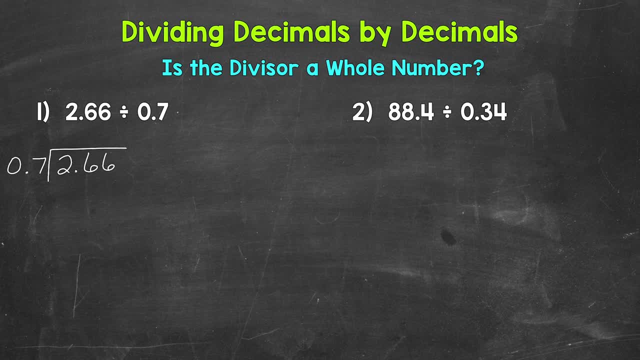 We can divide by 7 tenths. We can do this by moving the decimal once to the right. That will give us a whole 7.. Now, technically, we multiply our divisor by a power of 10. In the case of number 1,, 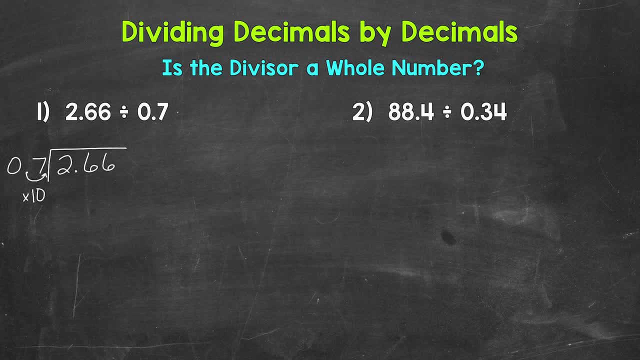 that power of 10 was 10.. So we multiplied 7 tenths by 10.. This shifts the digits of our divisor to the left and gives us a whole number. We made this process It's much simpler to think through by just thinking of this as moving the decimal to 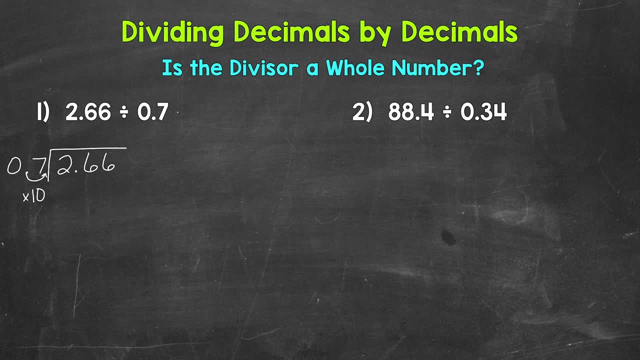 make the divisor whole. Now, whatever we do to the outside the divisor, we must do to the inside, the dividend, in order to keep this problem balanced and equivalent. So we need to multiply the dividend by 10 as well. Let's move this decimal once to the right. 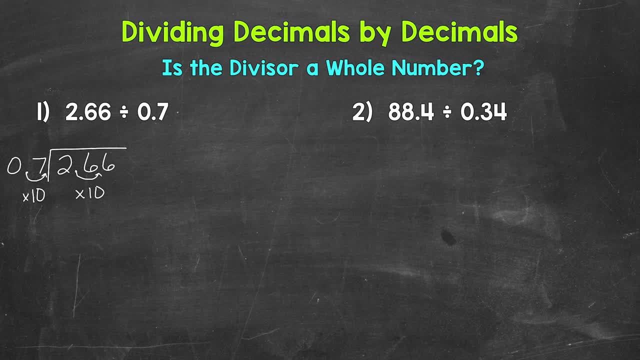 Now we can rewrite the divisor by 10.. We can do this by moving the decimal once to the right. Now we need to multiply the dividend by 10 as well. Let's move this decimal once to the right. Now we can rewrite our new equivalent problem with the whole divisor. 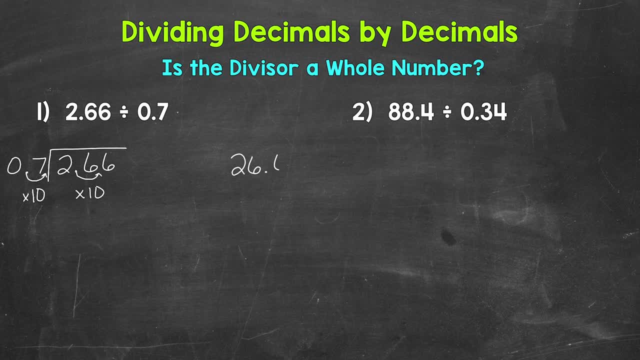 So we have 26 and 6 tenths for our dividend and then 7 for our divisor. So is our divisor now a whole number? Yes, So we can bring our decimal straight up into our answer and now go through the division process. 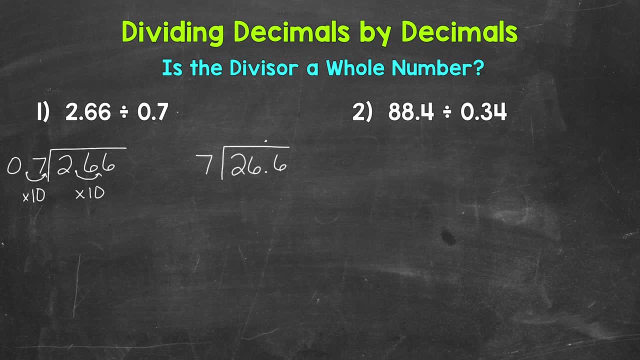 So divide, multiply, subtract, bring down, repeat. let's start with divide. so we have two divided by seven. how many whole groups of seven in two? well, we can't do that, so we need to use the six and take a look at 26. we have 26 divided by seven. how many whole groups of seven in 26? well, three. that gets us to. 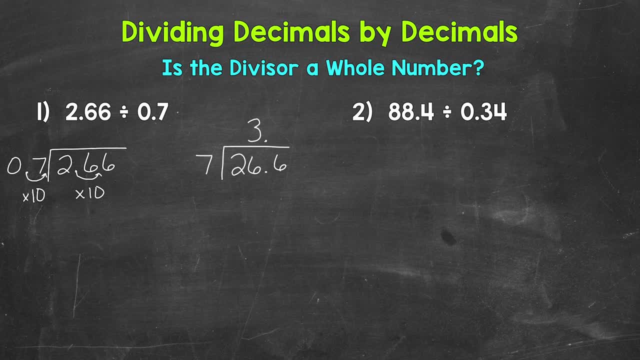 21. let's put the three above the six in 26, not above the two. it needs to go above the six, since we did 26 divided by seven. now we multiply three times seven is 21. subtract 26 minus 21 gives us five. bring down now we have 56 and we repeat. so we go back to divide. 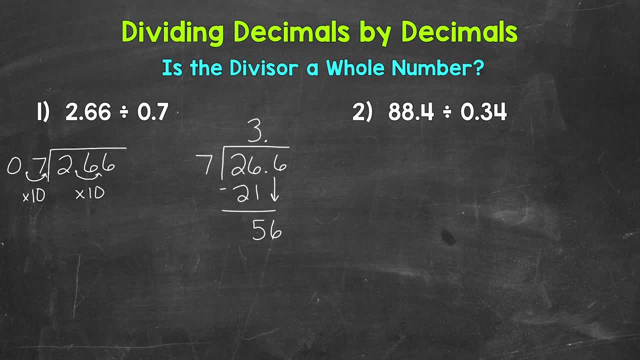 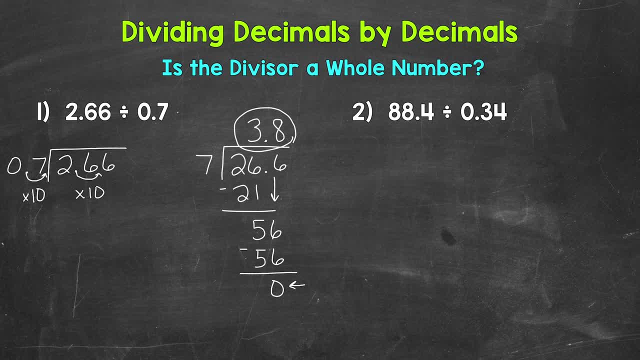 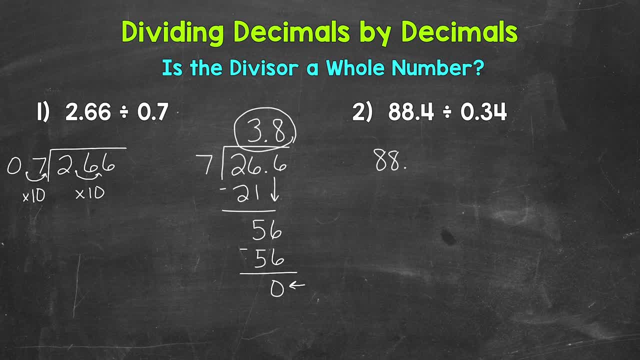